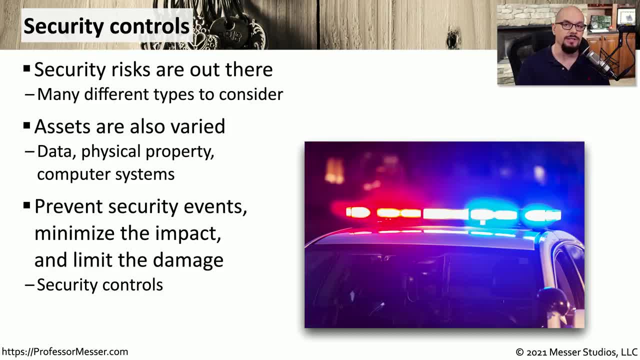 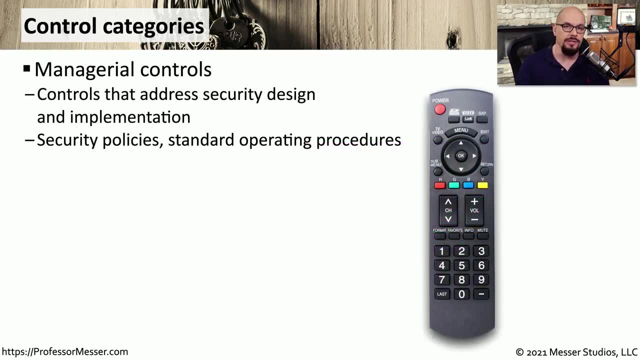 Our goals, then, are to prevent security events if possible, to limit the impact of any events that do occur and to limit any damage that might be caused. We're able to provide all of this through the use of security controls. We put security controls into three major categories. 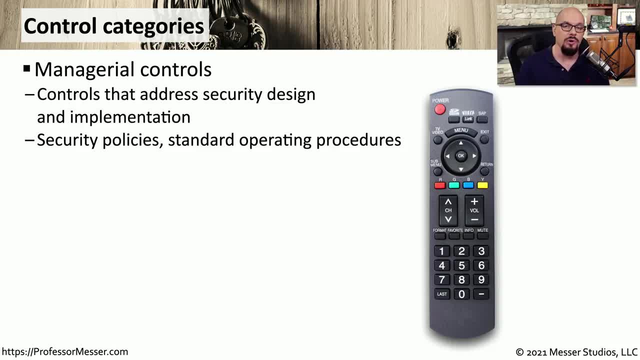 The first category is a managerial control. This is a control that focuses on the design of the security or the policy implementation associated with the security. So we might have a set of security policies for our organization or a set of standard operating procedures that everyone is expected to follow. 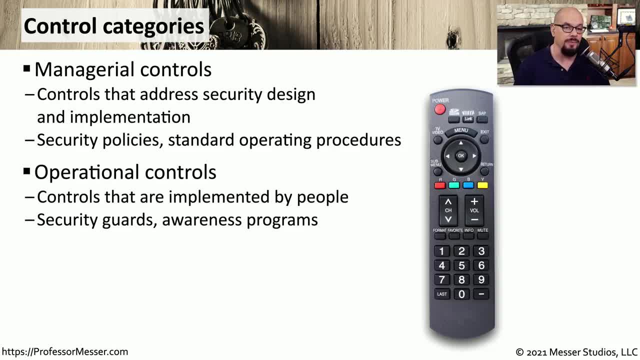 The second is operational controls. These are controls that are managed by people. so if we have security guards posted at the front doors or we have an awareness program to let people know that phishing is a significant concern, these would be operational controls And, of course, we can use our own systems. 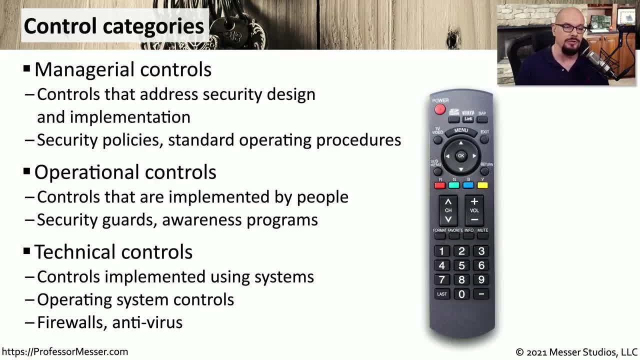 to prevent some of these security events from occurring. These would be technical controls. So if you've implemented antivirus on your workstations or there's a firewall connecting you to the internet, you would consider these technical controls. Let's now list some common control types. 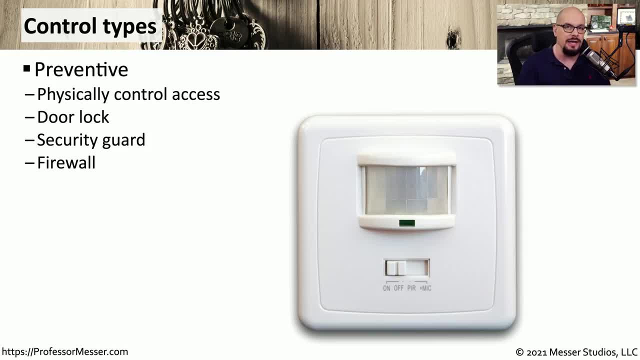 And what's interesting about these control types is a certain technology could fit into multiple control types, and you'll see that as we go through these. The first control type we'll look at is a preventive control. This would be something that prevents access to a particular area. 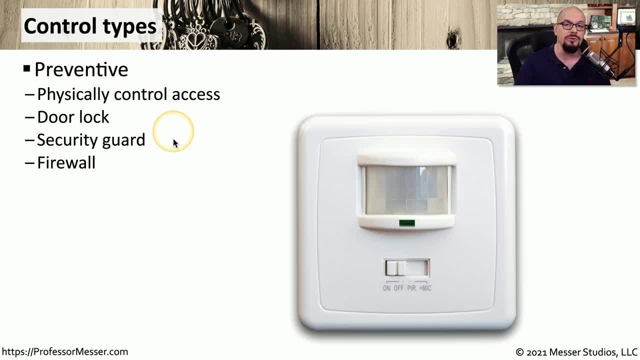 Something like locks on a door or a security guard would certainly prevent access, as would a firewall, especially if we have a connection to the internet. A detective control type commonly identifies and is able to record that a security event has occurred, but it may not be able to prevent access. 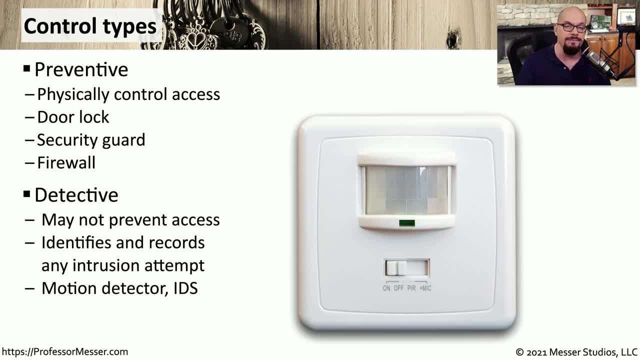 If you have a motion detector like this one, it can certainly identify that motion is there, but it's not able to stop someone from walking through the room. Same thing might apply to an IDS which is set to alarm or alert if it identifies. 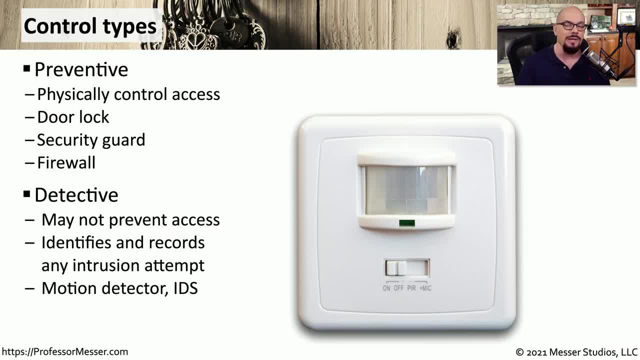 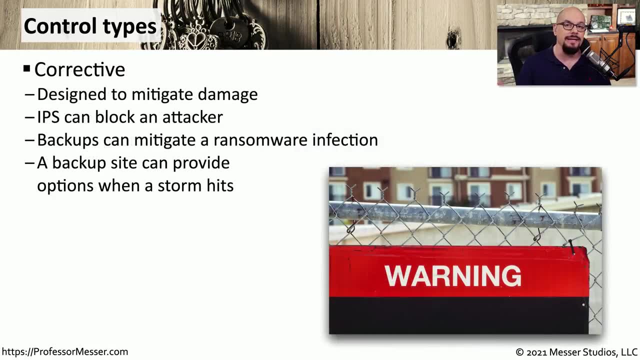 malicious software on the network. but an IDS is designed to only detect that traffic flow and not prevent that traffic flow. A corrective control is designed to mitigate any damage that was occurred because of a security event, For example an IPS, an intrusion prevention system.